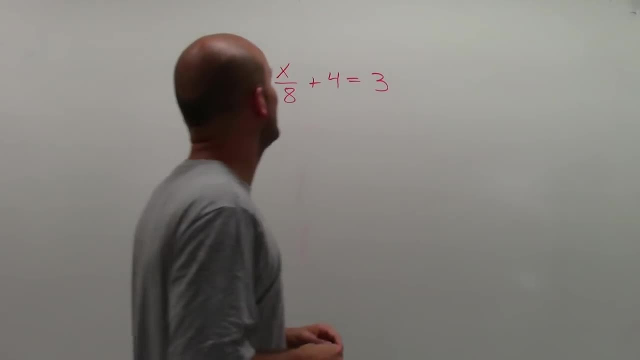 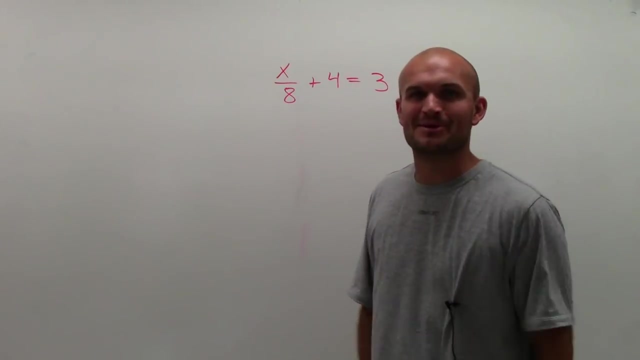 Ob-la-dee, ob-la-da. life goes on on on. life goes on. Sorry, I don't know. I'm just in a good mood today, so I was going to express it a little bit for you. Sorry, Here I have x divided by 2. 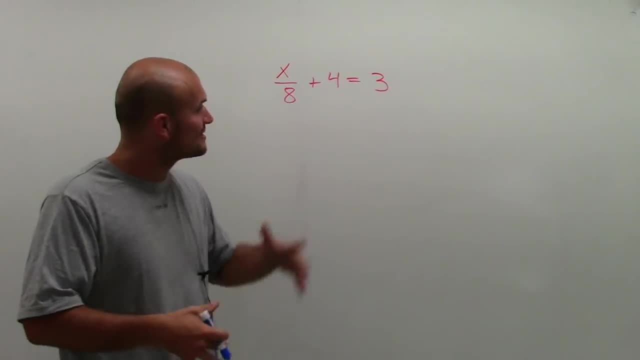 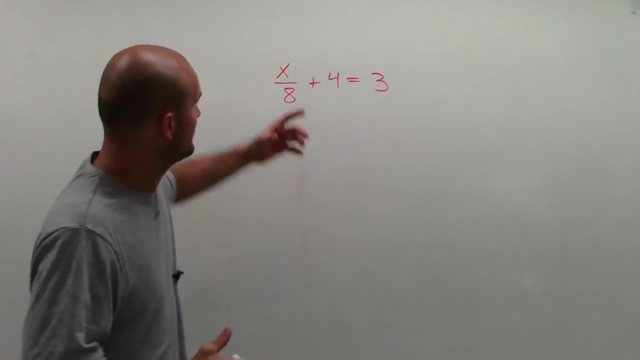 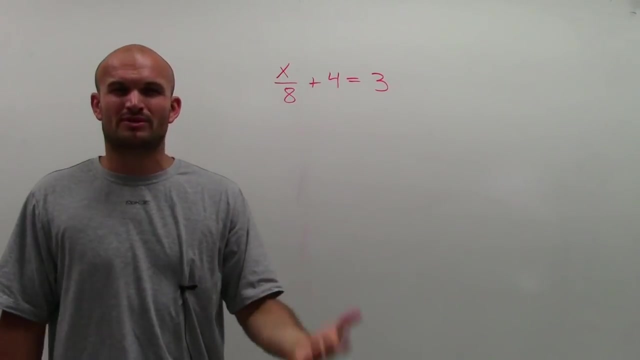 plus 4 equals 3.. So what we got to do is we got to solve this. And just remember, when solving two-step equations, we got to get our variable by itself. all right, We have our variable x, which is our unknown. We don't know the value of the variable And what value variable we're. 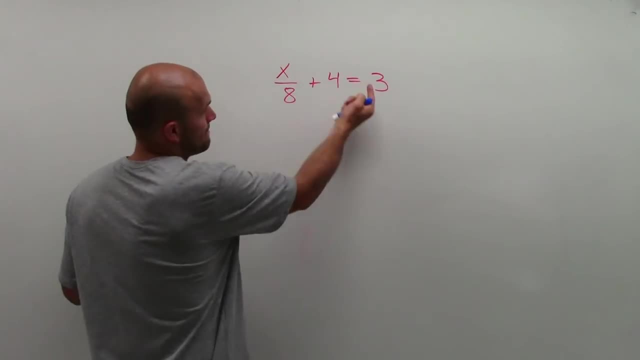 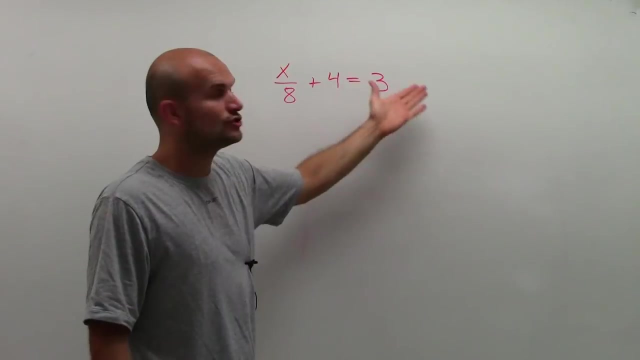 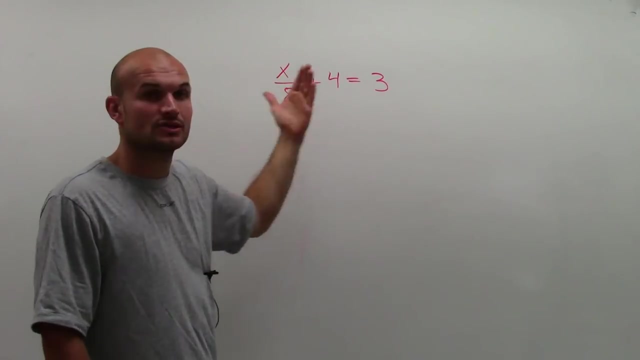 talking about is: I want to find the value of the variable that makes this equation true. okay, That means that this left side is equal to value to the right side. Well, the right side's value is 3.. So I need to find what value of x would make this true. Now you might be able to. 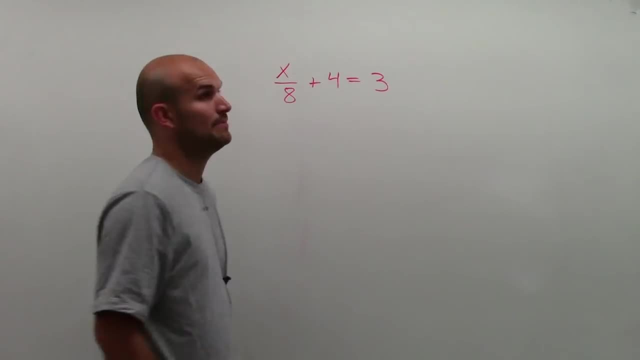 do this in your head. if you think about it, You could say: a number divided by 8, 4 equals 3.. So maybe think in your head, See if you can figure it out. However, I'll tell you you have to understand the process of solving two-step equations because I can throw out some 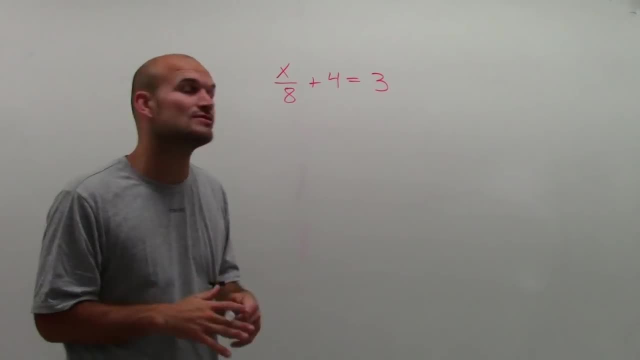 really crazy numbers out there that you wouldn't be able to do in your head that you're going to have to use this process to solve. So remember the first thing we need to do is undo addition and subtraction. So I look at my variable and say what am I adding or subtracting to my variable? 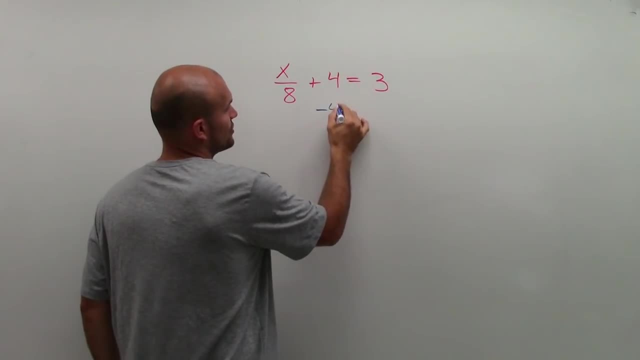 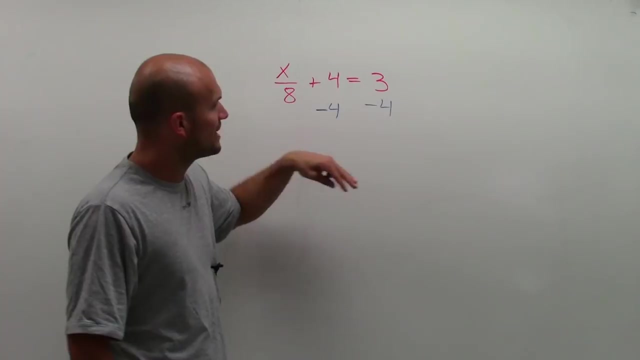 Well, I'm adding a 4 to my variable, so I'm going to subtract a 4,, 4 on both sides of the equal sign by using the subtraction property of equality. So, by subtracting on both sides, the left and right side have remained the same, what we call equivalent. 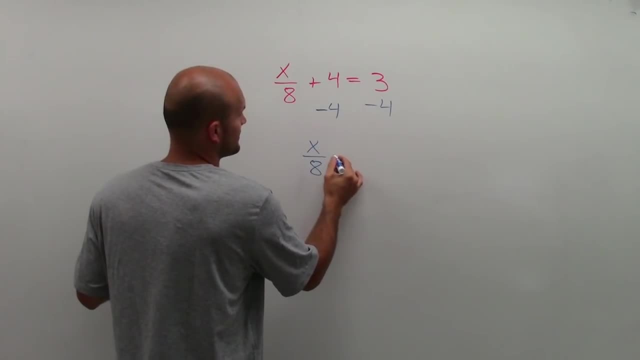 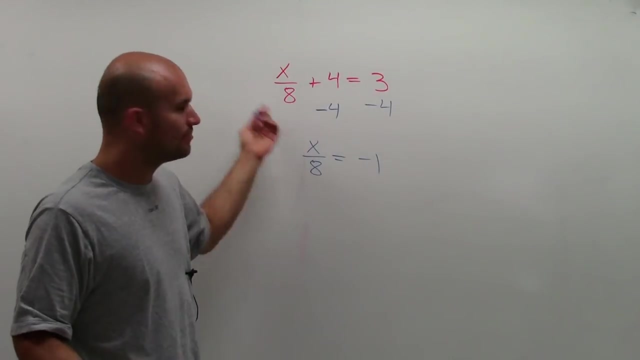 equations. So now I have: x over 8 equals 3 minus 4, is negative 1, because the positive 4 and negative 4 goes to 0,, 0 plus x over 8, still x over 8.. Now we take a look at my variable and say: